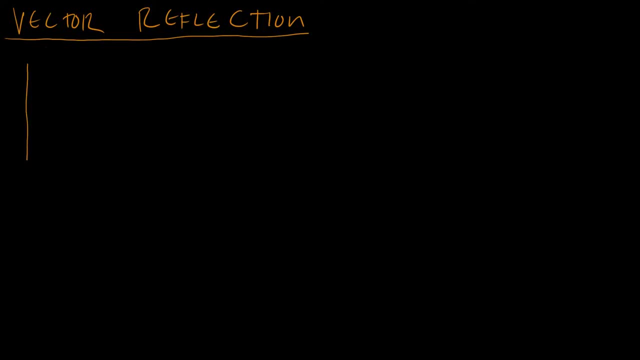 We now return to our regularly scheduled programming. I don't know what came over me. I just felt like doing a satire video. Hopefully I didn't embarrass myself too much. I probably did. So here we are. Let's say we're going to do a vector reflection problem. Oh, quick note before. 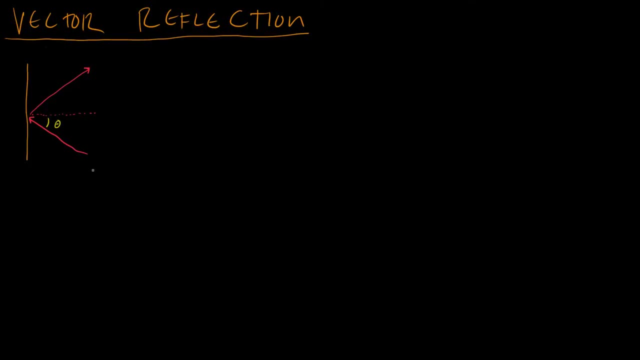 I get into the problem. This video requires some prerequisites, so you should have already watched through to the advanced matrices and advanced vectors playlists, because we need to know about some vector projections and about some coordinate spaces to do this video. So I'll have a link to: 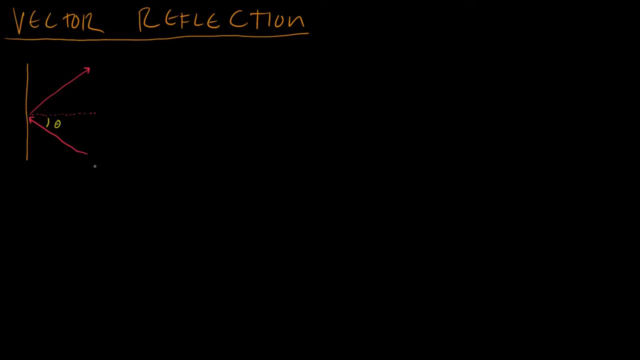 those in the description. Hopefully I won't forget. And if you haven't looked at those videos and there's something you don't understand in this video, then you can go to those videos and catch up. So, in any case, here's the problem. We have an object coming into a wall here. 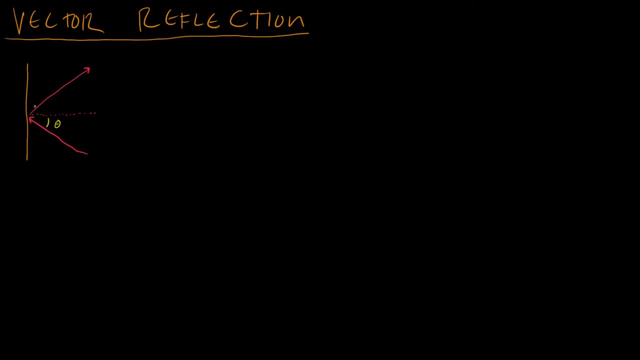 This is the red object And it's going to strike the wall and then it's going to bounce off at an angle such that the incoming angle that I've labeled theta here we want it to be the exact same as the outgoing angle, So it's going to be a perfect reflection And like the way it's drawn right now it looks, 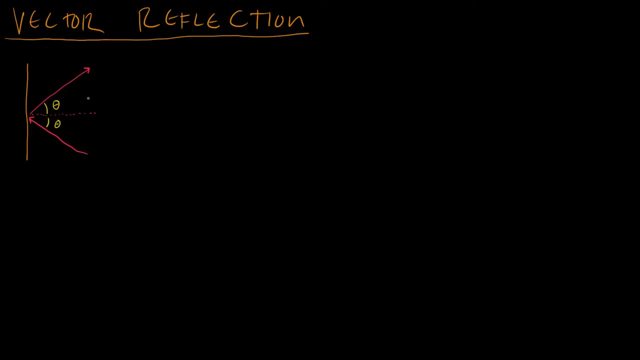 like a laser hitting a mirror. That's an example where you would want to make a perfect reflection. So you have a puzzle game where you have lasers hitting mirrors all the time, a puzzle game about lasers Then then you might want to do something like this, Or this happens a lot more often than 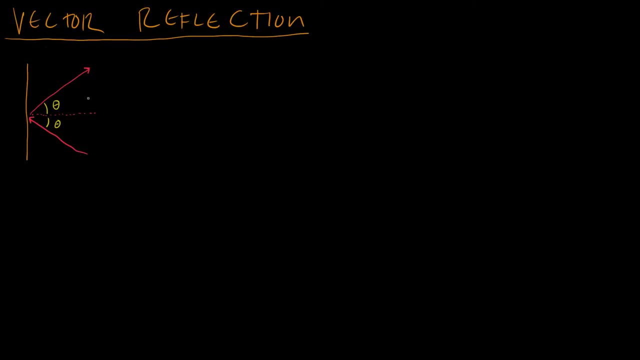 a lot in physics simulation. If you have an object striking a wall with a perfectly elastic collision- so for example, very bouncy ball hitting hitting a wall- then you would get a collision like this. You have to do this kind of a calculation So, so this comes up a lot in video. 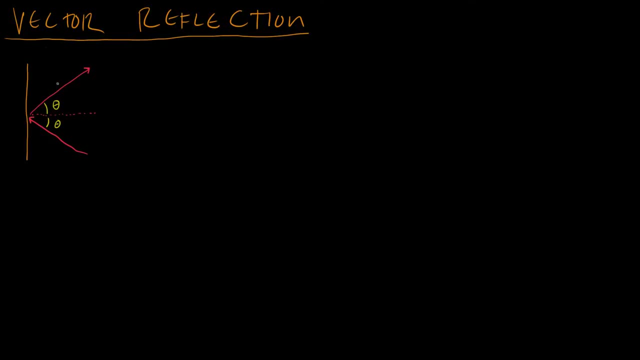 games. So we're going to study it today, how to reflect this vector against the normal of the wall. And I'm going to just give us the variables we have to work with. This is V, which is the vector that we are going to reflect, And this is n- doesn't even have to be unit length, which is: 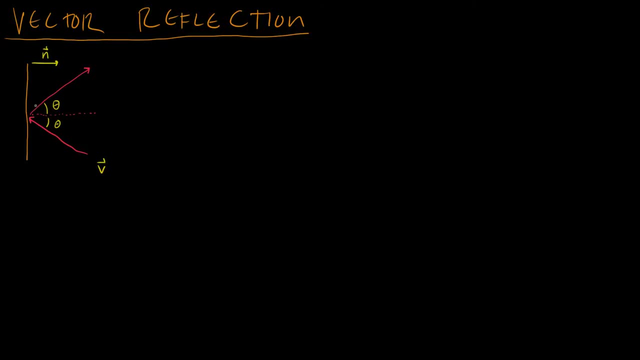 going to be the normal unit, the normal vector of the wall. So let's do a very simple case here. Let's assume that the x dimension and the normal of the wall line up perfectly, So the wall is in the wall and the normal of the wall line up perfectly. So the wall is in the wall and the normal of the wall line up perfectly, So the wall is in. 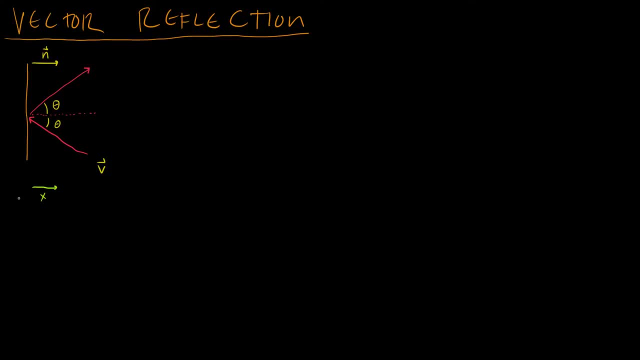 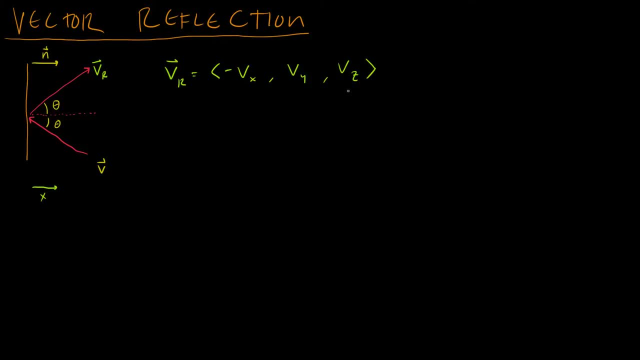 the way they are, and I mean, you can see that this is going to give you, if you, if you just look at it long enough, you can see that this is going to give you the reflected vector, because the vector starts here and it ends there, and we're 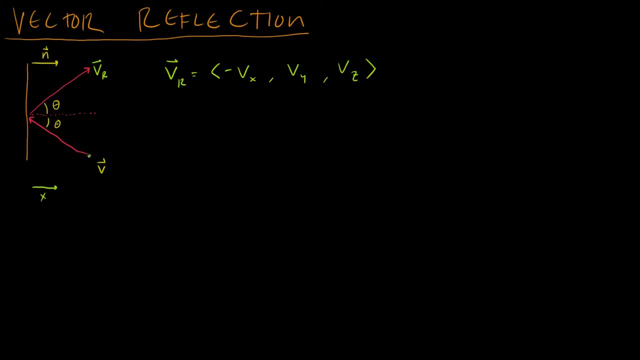 going to keep the up component the same. we're going to keep the Z component that goes into and out of the monitor the same, or Y, or however you want to consider. we're gonna keep those two the same, but we're gonna reflect the X component. so, instead of coming here, it's gonna go this way and we're gonna get a. 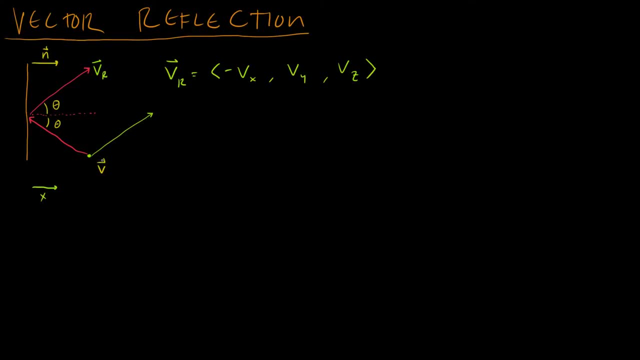 vector that points up here. now remember from our introduction to vectors course that a vector is a position, I'm sorry. it is a magnitude and a direction. it is not a position. so this vector and this vector have the same magnitude, they're both the same length and they have the same direction. they both point at the 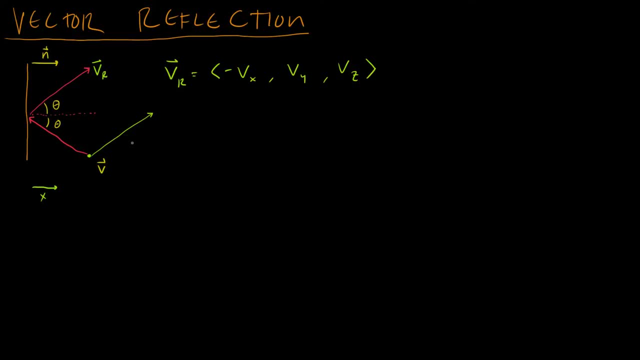 same angle and so they really are the same vector, even though they're in a different position. so this is VR as well. so in the very simple case that the normal is facing exactly in the X or Y or Z direction, this is a very easy problem to solve. but what if it's not? 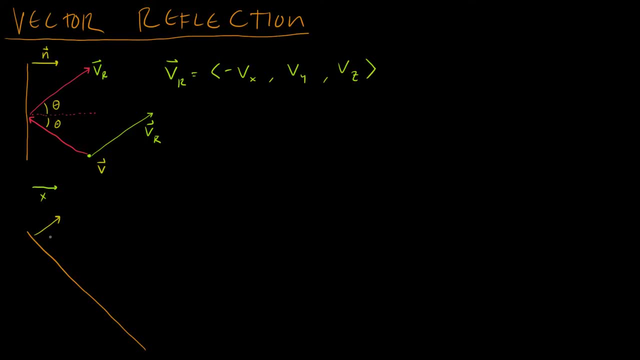 what if you have a plane that's facing at an angle like this- any angle really- then you have a problem. you can't just do this really easy swapping of the components like we just did. so if you can redraw it, that looks good. so we want to still keep these two angles the same. how do we do that again? 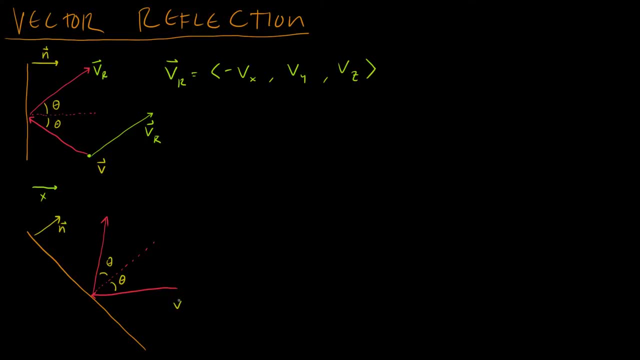 this is the normal vector and then this is the V vector that we're trying to reflect and it ends right there. so there are two approaches, and I'll first go over the more naive approach that has to do with coordinate spaces. again, you should watch the coordinate spaces video first, and that is to create. 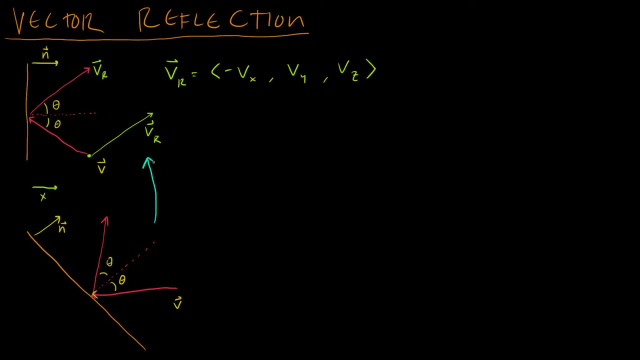 a matrix M that takes us from this coordinate space, where the wall is rotated, to a local coordinate space where the wall is not rotated, and when you do that you'll have a vector. M should not be a subscript, MV. okay, V is the vector in the global coordinate space and M is the vector in. MV is the. 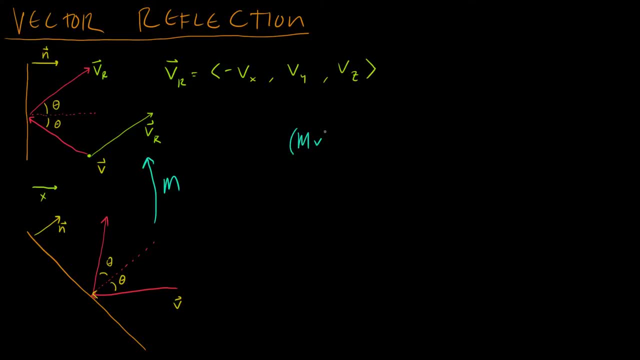 vector in the local coordinate space, this entire thing. MV is the vector in the local coordinate space. if all of this talk about coordinate spaces doesn't make sense to you, that's why I'm asking you: now is the time that you should go and watch the advanced matrices playlist. okay, so then all we 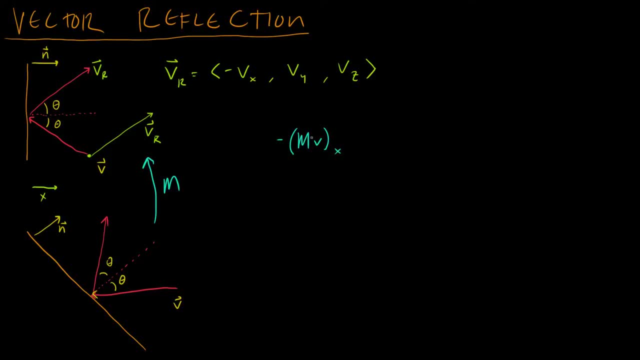 have to do is say: well, the negative, the negative X component of that vector, and then the Y component, and then the Z component, and we're going to build a vector same way we did before. now we have this vector and we're going to call that- what can we call it? V star, something like that. now, 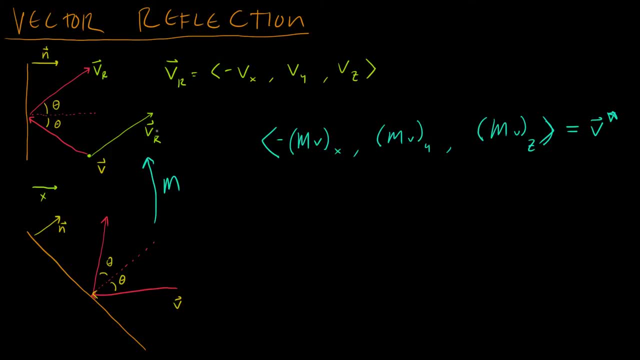 we're just going to come do this easy computation in the local space, that where we already know how to do it, and then we're going to go ahead and do this and then we have to convert it back to the, the global space, and we do that with. 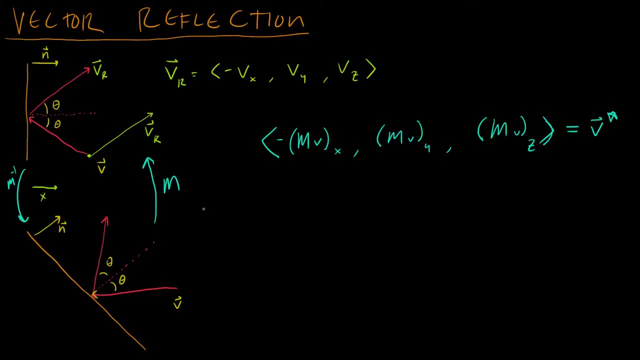 this M inverse vector, so we just say so. now we know VR is gonna be M inverse times this V star vector that we already calculated. so this is a great way to do it, except that it's not very satisfying to me because you have to construct this. 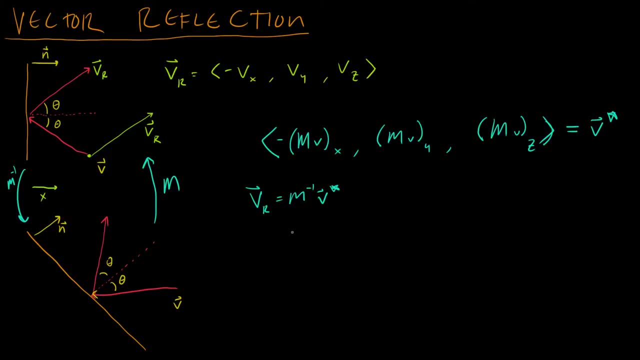 matrix, which we talked a little bit about how to do that in the in the advanced matrices video, but it's not straightforward. I mean you can do it, but it's it's not as easy as we would like it to be. and then you have to take the. 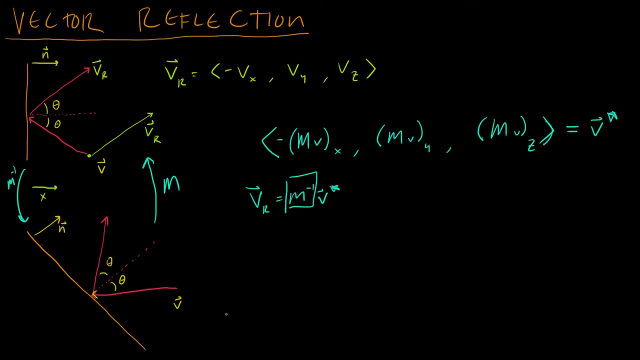 inverse of the matrix and that we try to avoid if possible. but it turns out we don't really have to do any of this at all. let's see how we can solve the problem with projections projections. we can solve the problem with projections. projections should have been the very last video that i did in the advanced vectors series, so if 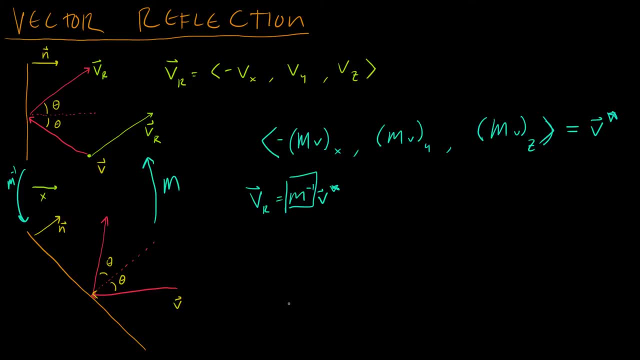 you don't know how to do vector projections. take a look at that right now. and vector projections are very powerful. we're going to see one way in which we can use them right now. so we're going to make an orthogonal projection here of v onto the normal vector. 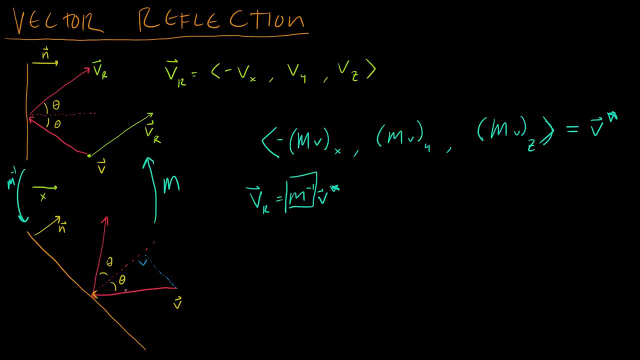 and i've drawn the normal vector here off to the side, but i may as well have drawn it right here, right, because again, moving a vector doesn't change what vector it is. so i just drew, i just stuck it right in there. now we're going to take this orange vector, okay, and we're going. 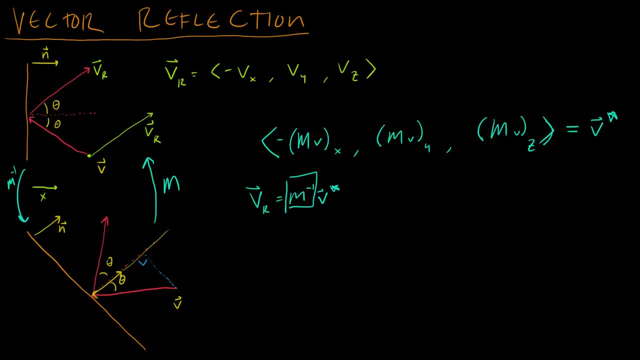 to project it onto the normal vector, and what will we get in purple- i will draw it very thickly. here we get a vector that looks like this: it starts right here, at the base of this triangle, and it continues until it meets with the original v vector. so this, right here is that. right there, that purple vector is v p. i'm going to call that. 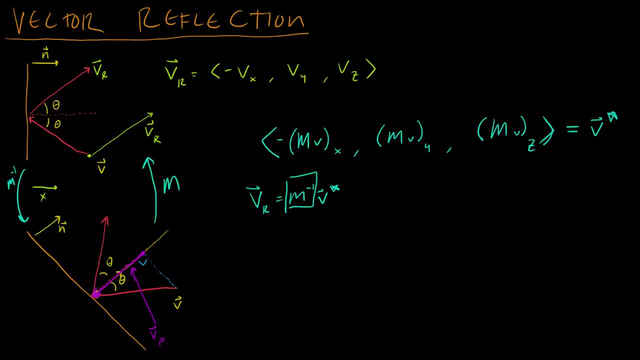 vp. that's a projected, that's v projected onto n. so don't forget: same as over here. this is what we want. we want this vr reflected vector right here. how can we build that out of the vectors that we have? we have v- it goes from here to here. and we have vp: it goes from here to here. well, what happens? 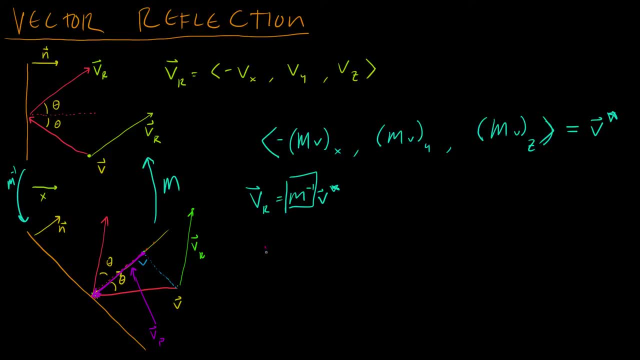 if i take v, okay, and then i subtract two of vp, i'll start here and i'll go to v and then i'll subtract a vp, so i'll end up here, and then i'll subtract another vp and i'll end up here and i'll get the vector that i want. so this is. this is the. 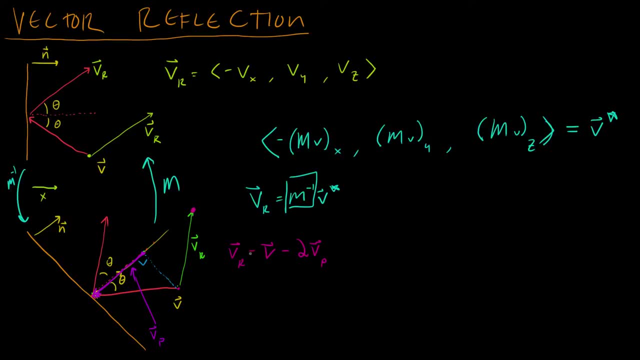 vr, that we want v minus 2 vp. now, if you remember from our video about how to do projections, this will be: this will be the projection onto n of v. okay, which now i'm going to substitute in the formula for a vector projection, which is v dot n over n dot n times n. again a very powerful formula which you. 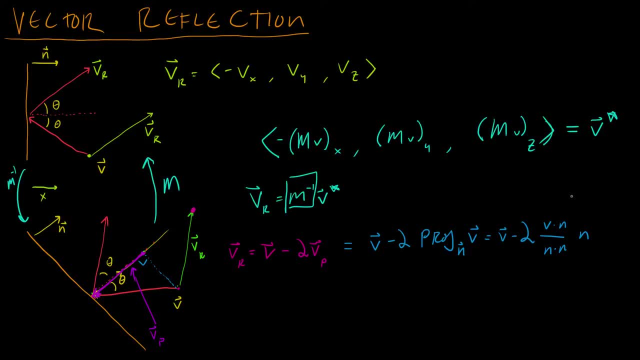 should commit to memory if you want to be a game developer, a game programmer anyway, because it lets you do so many things like this. uh, quick note: don't forget that if n is unit length, if you know that n is going to be unit length, then you can just cr n dot. n is one, so you can just cross that out there. we should have. 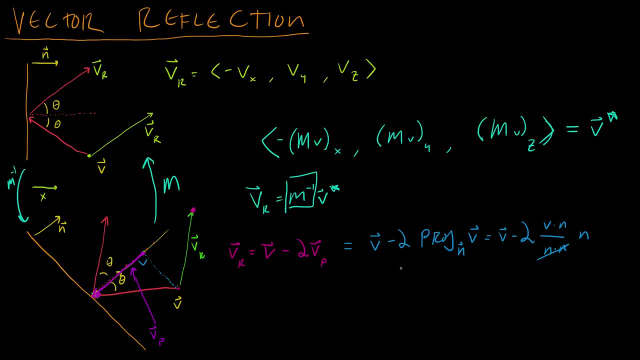 covered that in a previous video and so that's it. i'll write it again in a nice bigger and a nice brighter color so it's easier to see minus 2 v dot n over n dot n times n, and that will be this vector right here now. the last step is figuring out what's going to be the vector that we want to.